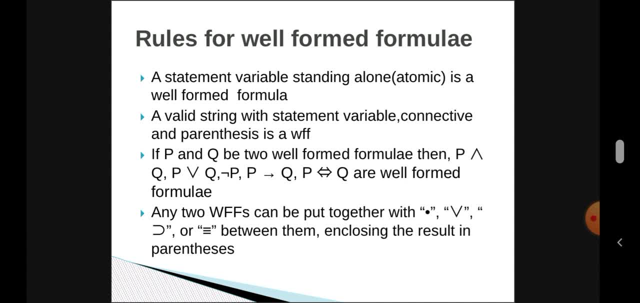 A statement variable standing alone or we can say atomic is a well-formed formula. And the second one is a valid string with statement variable, connective and parenthesis is a well-formed formula. And if P and Q be two well-formed formulae, then P and Q, P or Q, negation P, P implies Q etc. are well-formed formulae. 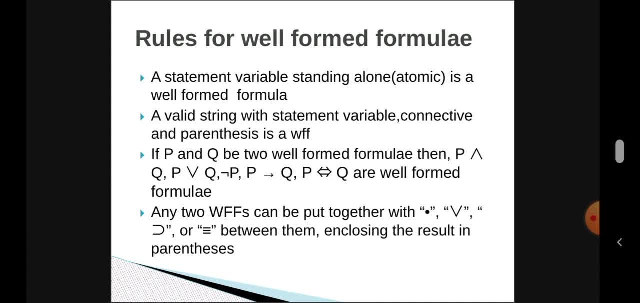 Any two well-formed formulas can be put together with dot or and. Etc. between them and closing the result in parenthesis. 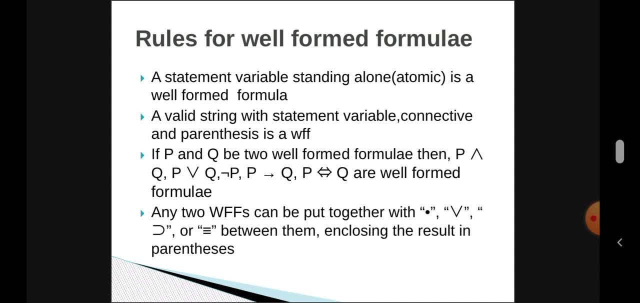 So, a well-formed formula is a well-formed formula that follows syntactic rules. So, it has certain rules. What are the rules? 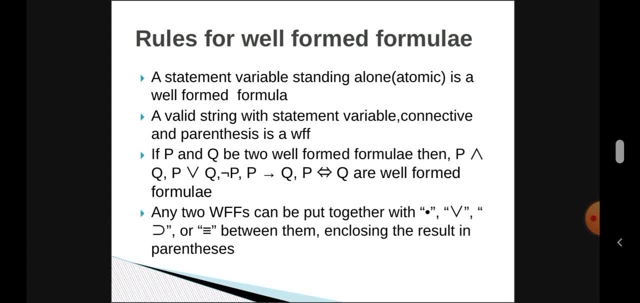 There are two types of statements, atomic statement and compound statement. 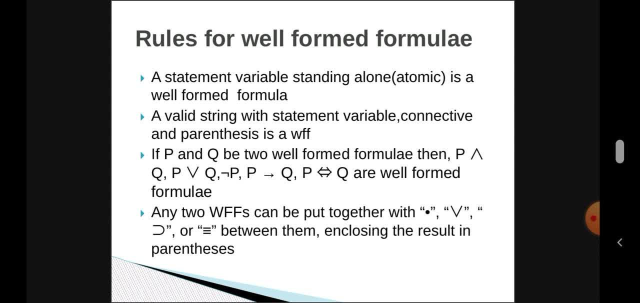 Atomic statements are capital letters, P, Q. Single letters. So, single letters are simple letters. We call it atomic. 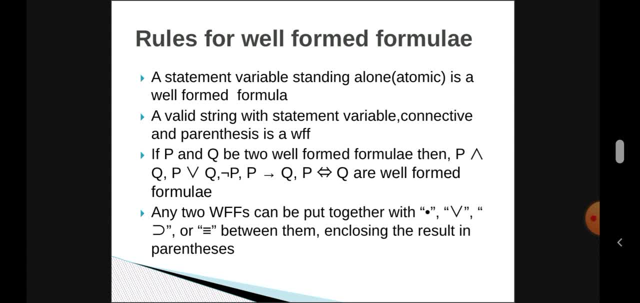 So, a variable standing alone. So, that is what is in a well-formed formulae. Okay, next one. 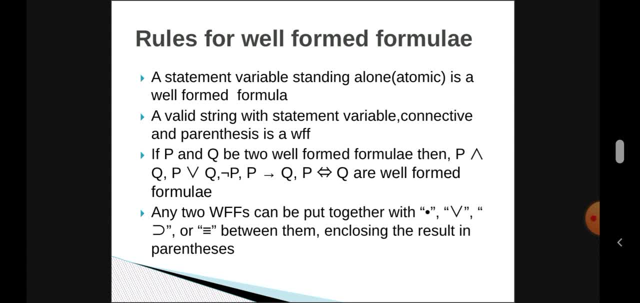 We can use a variable using a connective or parenthesis. So, this is a well-formed formulae. 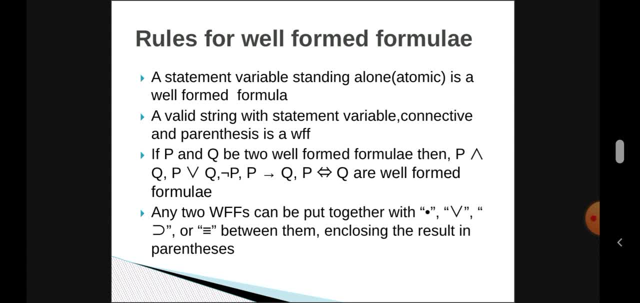 Okay, then next one. So, P, Q. If these two are well-formed formulas, then P and Q, P or Q, negation P. 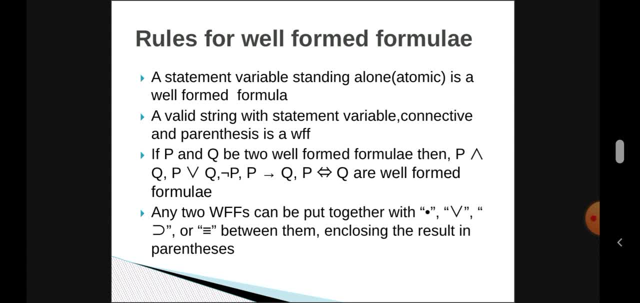 All the sequence of strings using connectives like this. Okay, or statements. Sequence of statements, we can say in another way. That is also a well-formed formulae. Okay, this is what I said earlier. Any two well-formed formulas can be put together in dot or and. 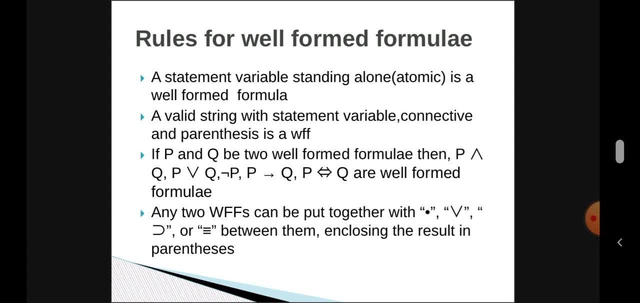 Put together in dot or and etc. Then enclosing the result in parenthesis. We can use a parenthesis for such expressions. That parenthesis is a bracket sound. 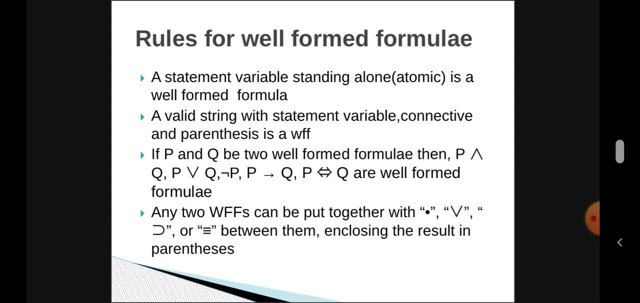 So, this kind of parenthesis is aligned correctly. If there is a left parenthesis, there will definitely be a right parenthesis, a closing parenthesis. So, this statement should be well-formed in that way. Okay. 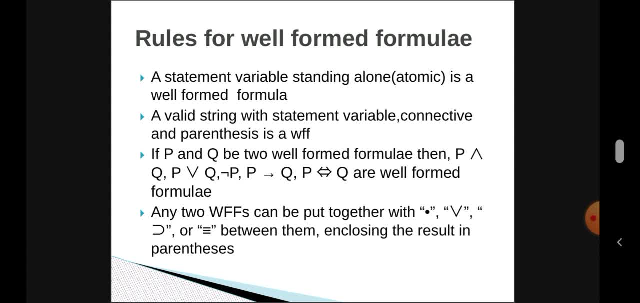 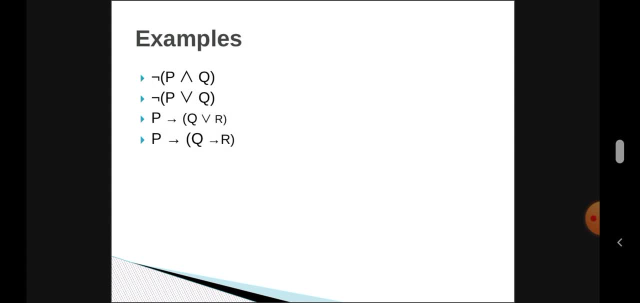 So, what are the statements that follow these rules? What is a well-formed formulae? For example, negation of P and Q. 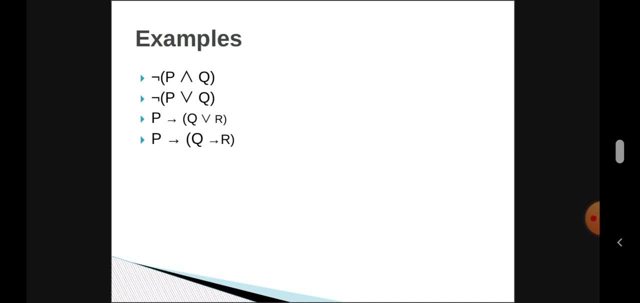 Negation of P or Q. P implies Q or R. Or P implies Q implies R. 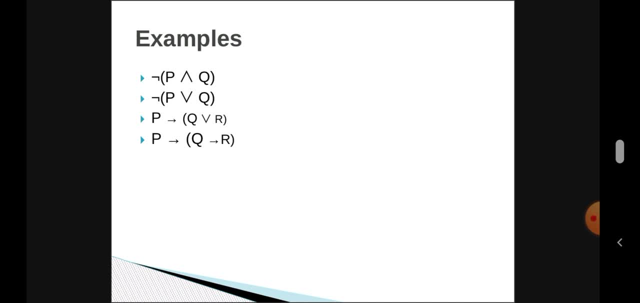 What are all these? These are all the examples of well-formed formulas. Because we have arranged in the right way. Okay. 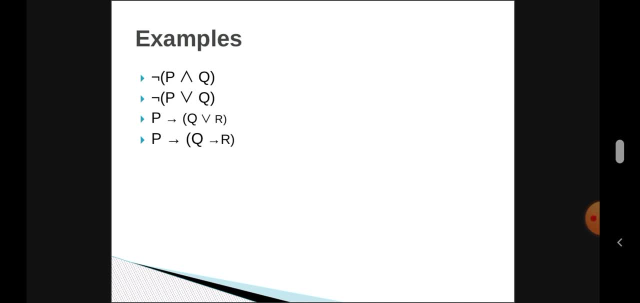 So, when we say negation of P and Q, there will definitely be a left parenthesis or a closing parenthesis. So, if there is an opening parenthesis, there will definitely be a closing parenthesis. Okay. 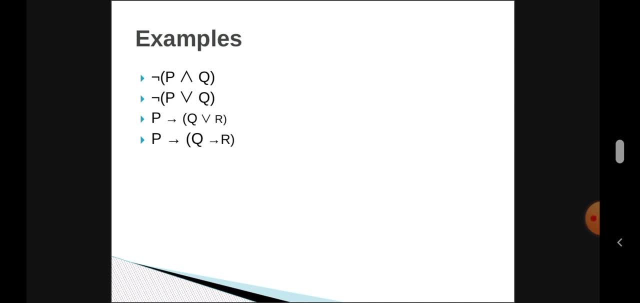 Similarly, how do we arrange it? Negation is arranged before any statement. Okay. 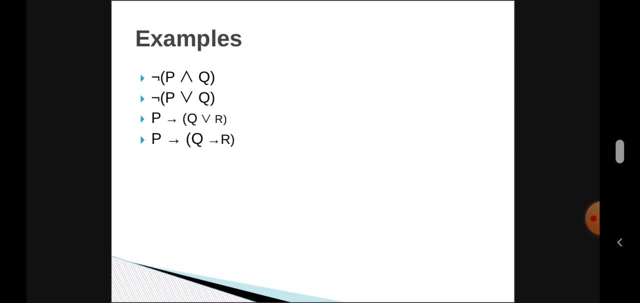 So, we should follow all these well-formed formulas. Let's see those who are not a well-formed formulae. Okay. P and Q. Here, not matching parenthesis. 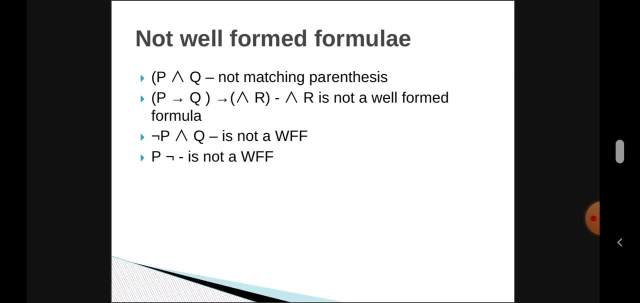 Here, we have a left parenthesis. But the closing parenthesis is missing in the first case. 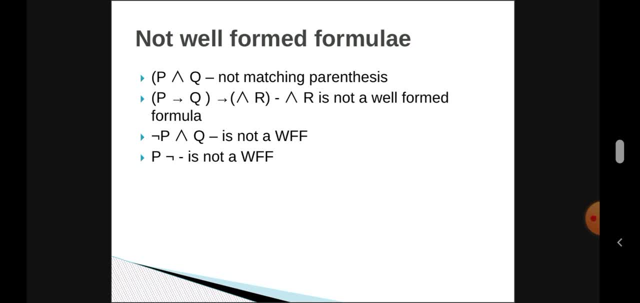 And let us see the second one. Here, P implies Q implies and R. 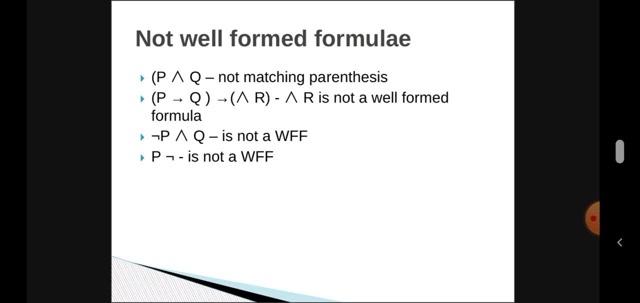 So, and R is not a well-formed formulae. We are expecting a statement before that, right? 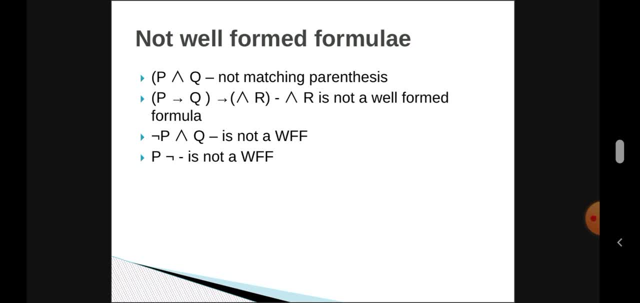 So, we can use this connective in between the statements. So, here the left statement is missing. So, this is not also a well-formed formulae. 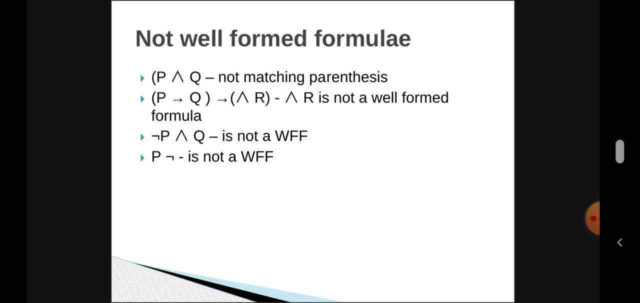 Next one. Negation P and Q. This is also not a well-formed formulae. 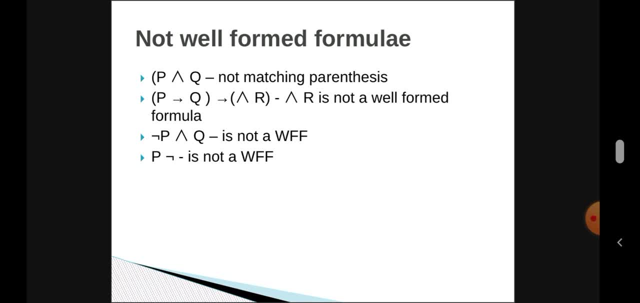 Because there should be a left and right parenthesis. Next. 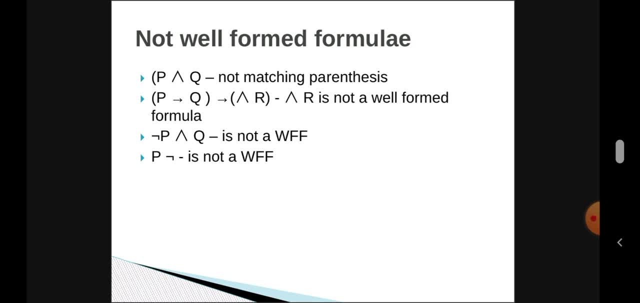 P negation. That is also not a well-formed formulae.